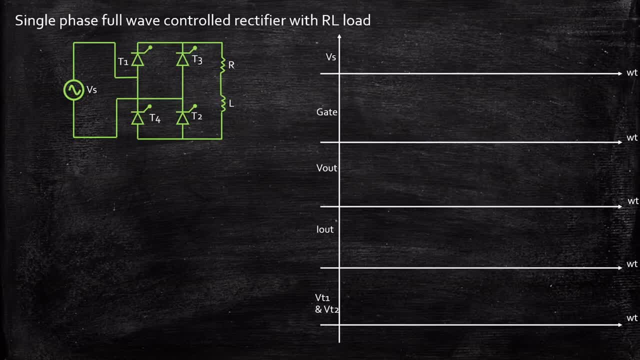 during different cycles and it will be very easy for you to understand. We are going to look at supply voltage, waveform, the gate pulse, Vout, voltage across the output and the current across the output, Iout, and voltage across thyristor T1 and T2.. One important 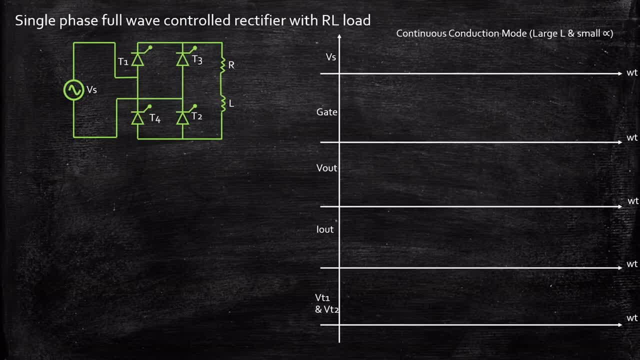 observation here is that we are going to understand the operation of this circuit in continuous conduction mode. When I say continuous conduction mode, the output current will be continuous and it will never go to zero, and that can be achieved through large value of inductor. 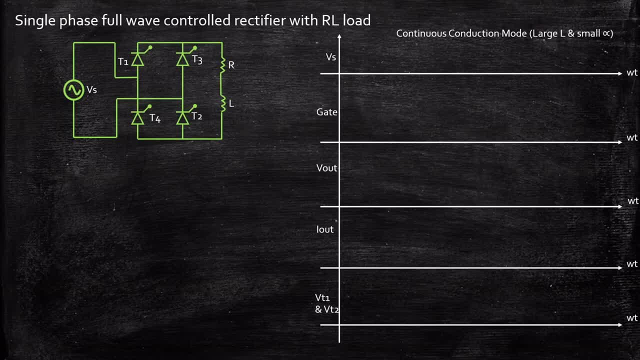 and small value of alpha, by designing the inductor such that the output current can be made continuous, that is, by large value of L and small value of alpha. We are going to consider a sinusoidal voltage source, Vs. Let us extrapolate these waveforms and let 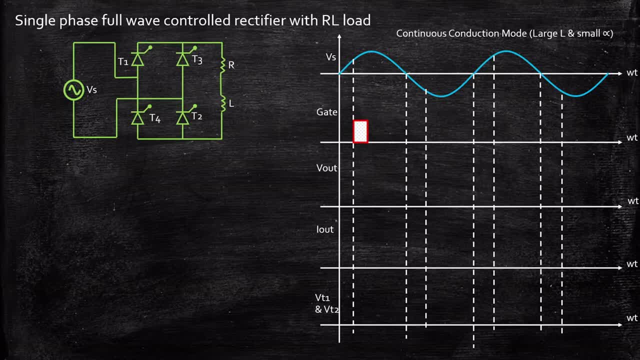 us understand what happens when we apply a gate pulse to thyristor T1 and T2 at, say, instant alpha. So T1 and T2 is triggered at instant alpha over here. So during this instant, what happens is that we will consider the circuit, So the supply voltage is going in the positive and 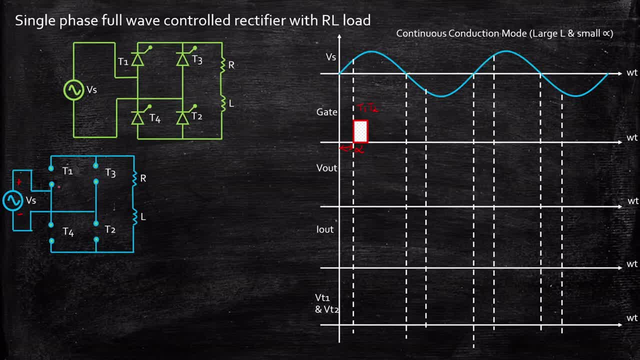 negative direction over here. Positive will be connected to anode of T1 and negative is connected to the cathode of T2.. Because of this- and firing pulse is applied at instant alpha, T1 and T2 will be acting as short circuit and T3 and T4 will act as short circuit. So 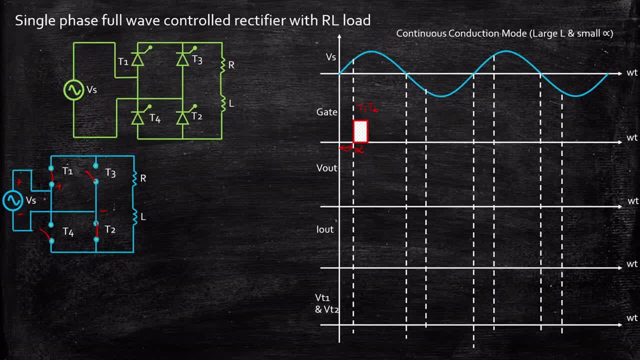 the current starts flowing through this path. The current flows through this path, The current flows through the load in this direction and the current flows through this path. It returns to the source in this particular direction. Meanwhile, one important observation is that the output voltage is plus and minus because 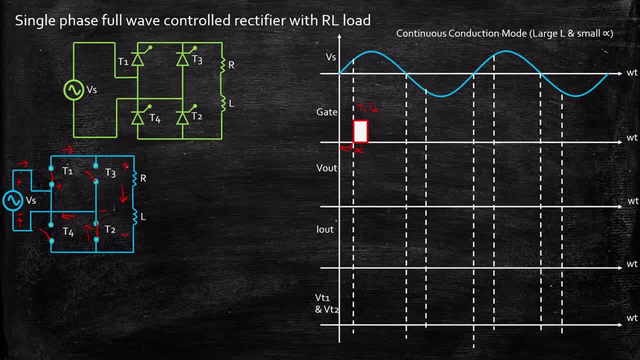 the current is flowing from upward to downward direction, So we have considered this as the convention. One important point here is: the inductor starts charging with a polarity plus and minus during positive half cycle. So what is the output voltage during this cycle? Vout is equal to Vs, because it is just 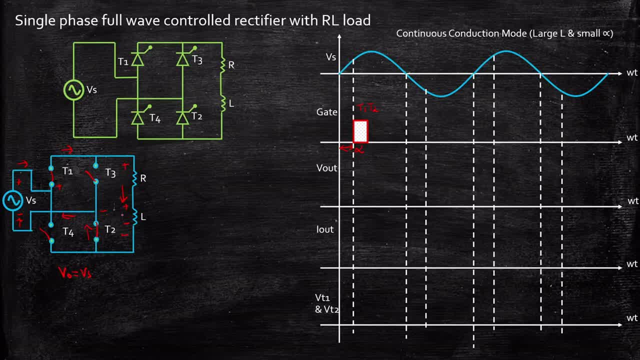 acting as short circuit. The current is flowing through this path and there are no power consuming elements apart from the load in the network, isn't it? So whatever you are supplying will appear at the load terminal. So Vout will be equal to Vs. So what is the output voltage? 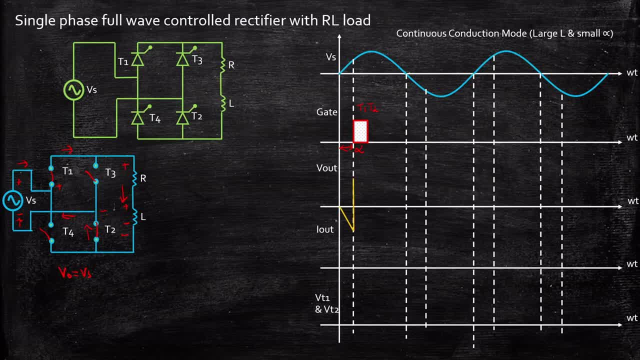 waveform, So the output voltage waveform will start in this particular fashion. I will tell you the reason why it is starting from this point. It is going in the negative. I will explain that in detail as we go ahead. But let us say when alpha is given, at this instant we 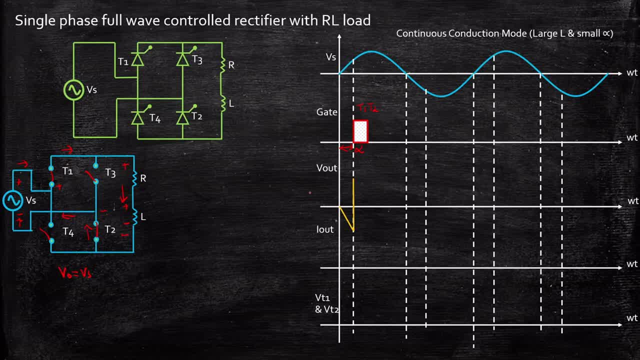 see that T1 and T2 is turned on. As a result we are having: Vout is equal to Vs, So Vout will basically follow the supply voltage waveform. So you will be getting a waveform which is similar to the supply voltage. 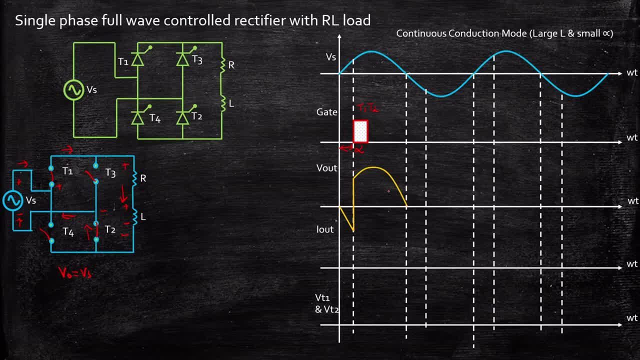 In this particular fashion. this is because of T1 and T2 conduction And what happens to the current? Again, I will be explaining the dip, the reason for this dip. as we go ahead At this instant, what happens is that the inductor starts slowly charging As a 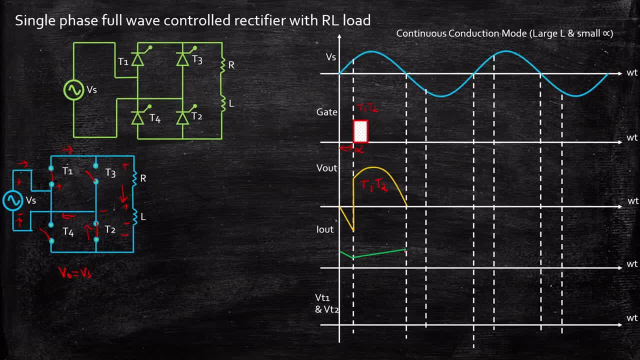 result: the current slowly starts to increase and it reaches a peak value over here. Now, when negative half cycle appears, that is when supply voltage goes negative, what happens here? It becomes minus n plus. So we would have thought that T1 and T2 should be reversed. 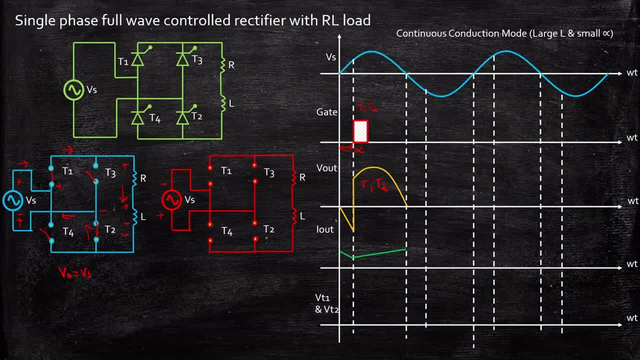 past, in this case, because negative half cycle has started, isn't it? But that is not the case that is happening. So what actually happens is, according to the property of Lenz law, the inductor will reverse its polarity as minus n plus, and it will ensure that the current 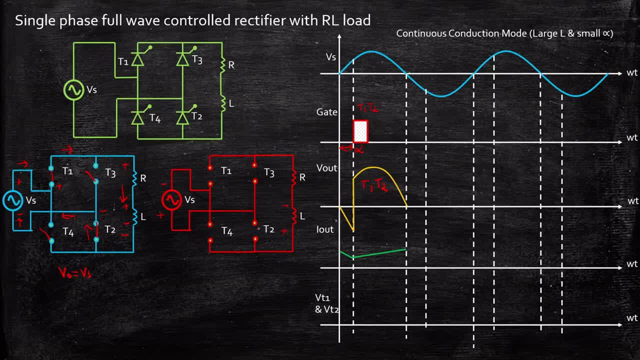 still flows in the same direction And, as a result, T1 and T2 will still be acting as short circuit for some time And Vout will be equal to Vout. So the current direction will be same as it was in the previous cycle. So we will be having 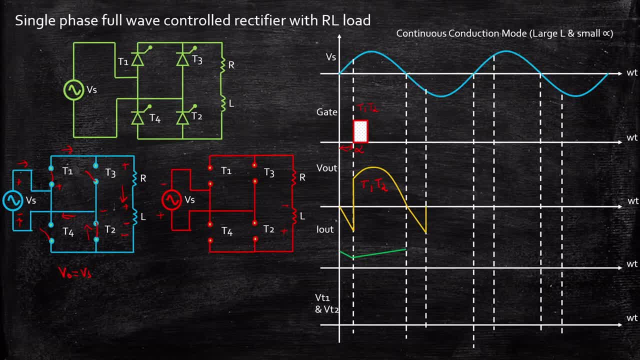 the output voltage waveform like this: It is still following the supply voltage waveform, So it is in the negative direction over here, And this is because T1 and T2 is still conducting. That is, T1 and T2 is still conducting And that is why we are getting this waveform over. 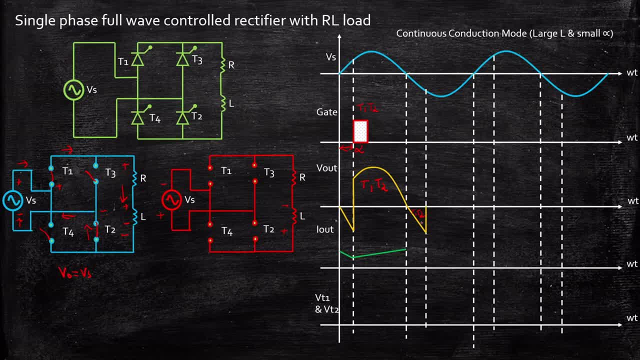 here And that is why it started like this. I just wanted to explain that, So I hope. why we are starting like this? because there was previous cycles, So it is starting at this point And now, when we are applying a gate pulse, similarly, the 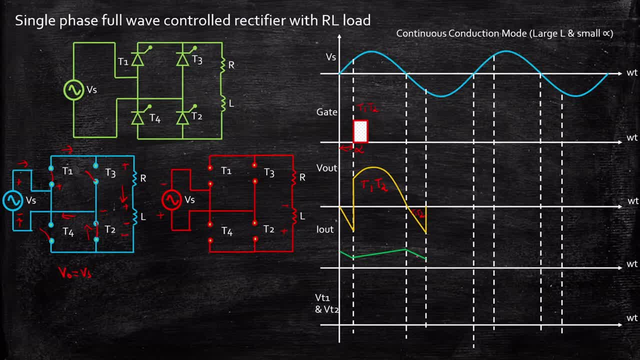 same thing happens to current. Why the current is decaying. The current is decaying because the energy in the inductor is getting dissipated and it is discharged through resistor R And that is why it is dissipating. And please note that the current is not going to zero. 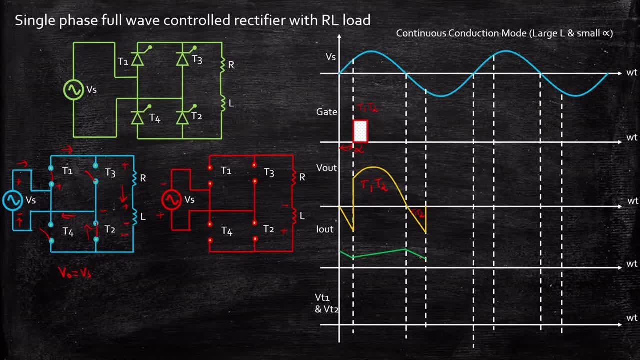 and it is having some value based on the inductor that is chosen. So that is never going to zero. if you carefully observe Now, when we are applying a gate pulse to T3 and T2, we can see that T3 and T4, what happens is that T3 and T4 will be turned on because plus is. 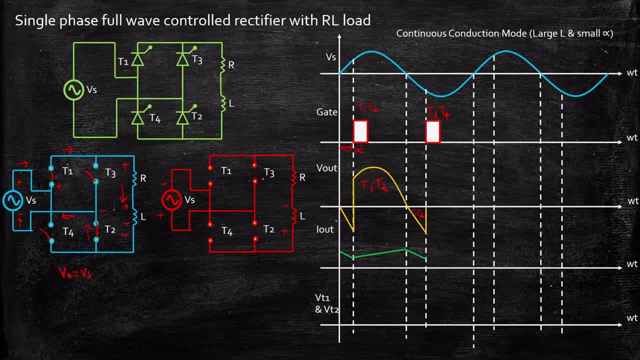 applied across the anode of T3 and minus is applied across the cathode of T4. These two will act as short circuit and this will act as open circuit. T2 also will act as open circuit, So the flow of current will be through this path. It will be through this path and 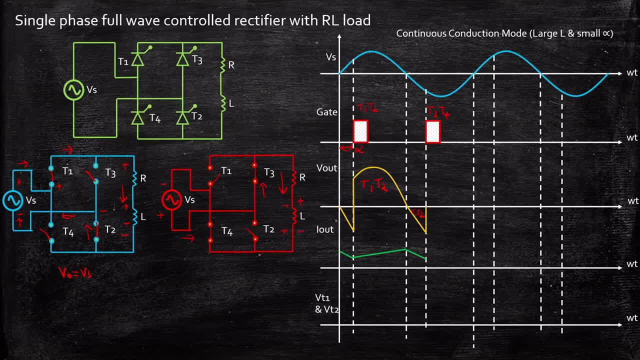 it will be through this path. Again, the inductor starts charging with a polarity plus and minus and the flow of current will be through this path And it will be through this path and it will come back to the source. So again, Vout will. 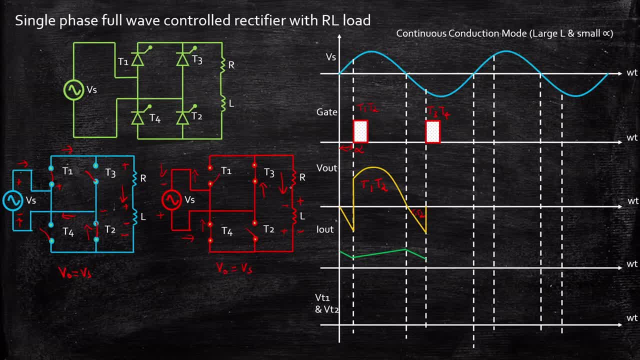 be equal to Vs. That is, Vs in this case is again positive and you will be getting a positive output voltage over here, meaning to say that the supply voltage will still have the same pattern of the waveform that we got in the previous cycle, That is, T3 and T4 is turned. 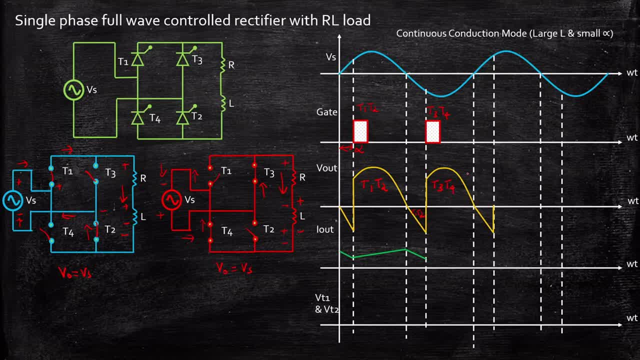 on And again when the supply voltage is in this positive direction, that is, it is in the opposite direction for T3 and T4. So the supply voltage will be in the opposite direction for T3 and T4. And again when the supply voltage is in this positive direction. 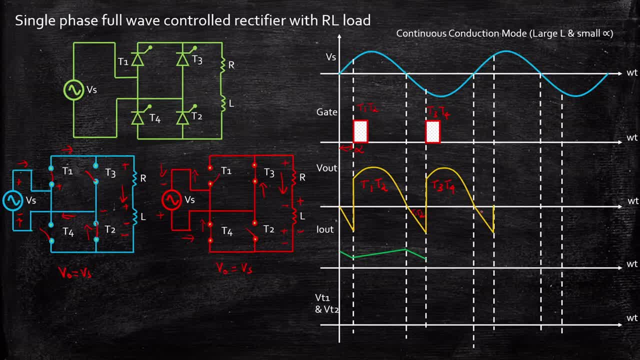 that is, it is in the opposite direction for T3 and T4. So what happens? It will still continue to conduct because of the stored energy in the inductor, as that was the case for T1 and T2.. So it will still conduct because of T3 and T4. The same cycle repeats for the 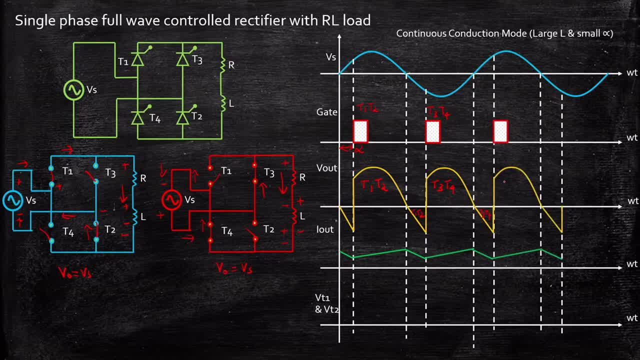 current waveforms and it continues to conduct because of T1 and T2, here and here T1 and T2.. So this waveform repeats for n number of cycles And, if you carefully observe, both positive and negative cycles are combined. These cycles are completely controlled with the help of a fully controlled rectifier. 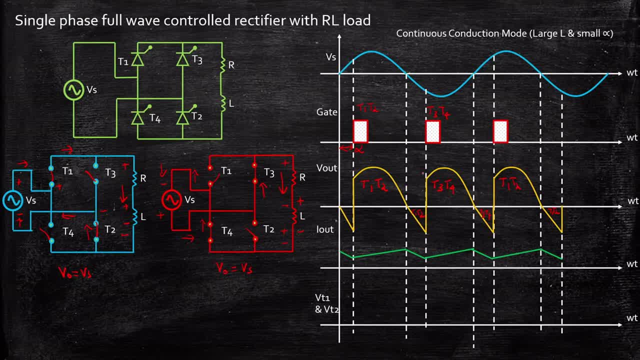 So full wave control rectifier controls both positive and negative half cycles to convert AC to DC. As a result, we call this as full wave control rectifiers. Now let's take a look at the voltage across thyristor T1 and T2.. And I would suggest you to try it for. 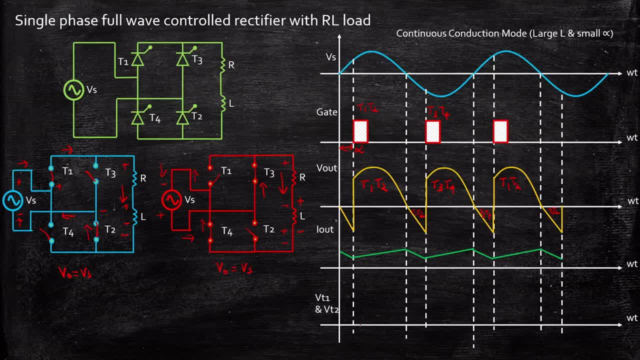 T3 and T4, because it is opposite to T1 and T2.. And that is why I'll only be showing T1 and T2.. So it starts through this peak. So again this peak, why it is starting like this. I. 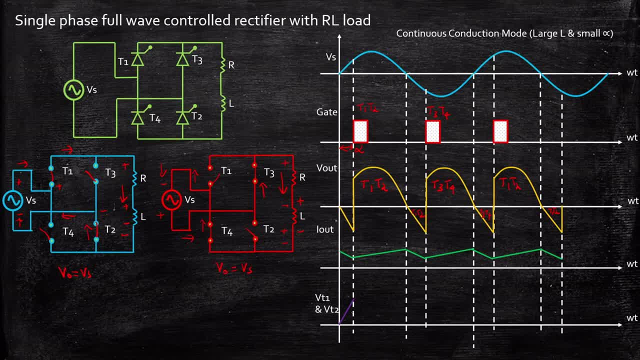 will explain further. Now. when T1 and T2 is turned on, the voltage across it will go to 0, isn't it? Because it is acting as short circuit. So it is going to 0 and till the instant when it is continuing to conduct, it will be in 0 only. So T1 and T2 will stop. 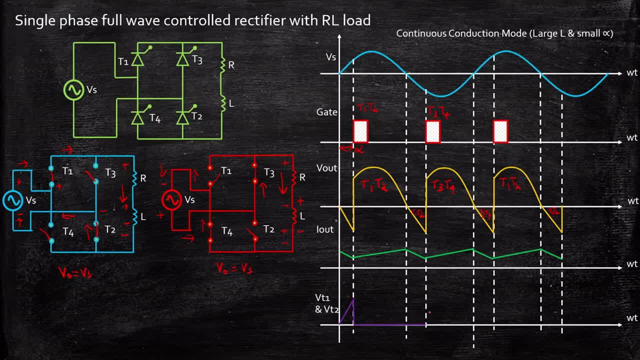 conducting. at this instant, And at only at that instant, you can see that the voltage across the thyristor will go and follow Whatever is the supply voltage. So it will follow whatever is the supply voltage. The reason is because it is acting as reverse biased. and when it is acting as reverse biased, 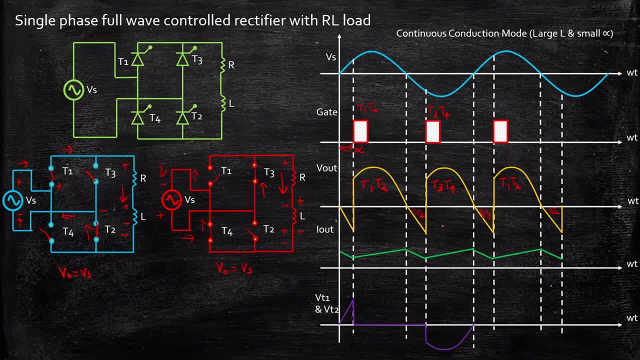 negative voltage will be applied across T1 and T2.. As a result, it is following the supply voltage waveform. I hope this point is clear. Now, again, now again. the cycle repeats, So you're getting a peak like this, And that is the reason why I'd shown this is starting. 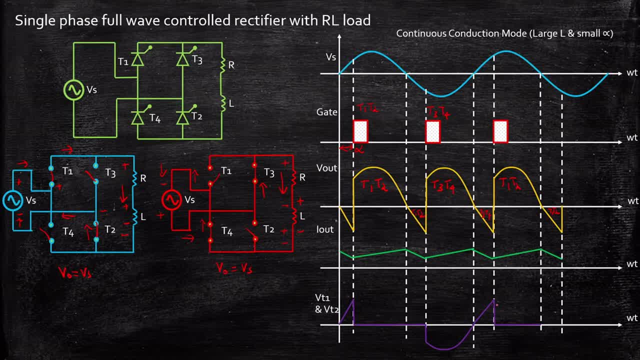 like this at this instant. So this pattern actually follows this, And when again T1 and T2 is turned on, it will go to 0 over here. So this is how you need to understand and analyze the operation of a single phase full wave control rectifier. Now let us take 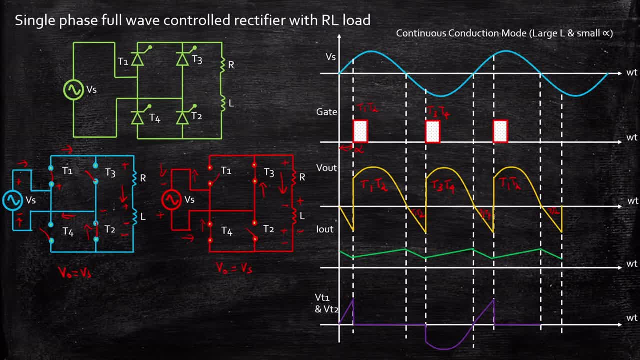 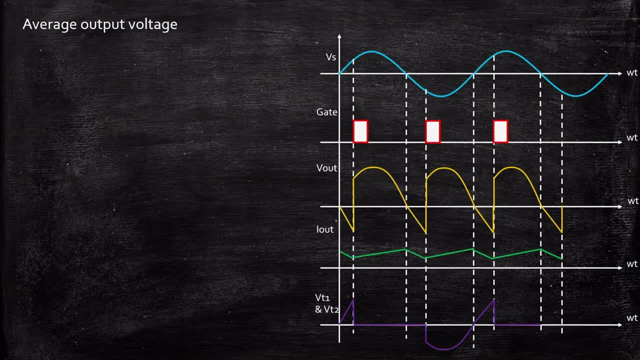 a look at some of the important analysis that we need to take into consideration. Now let's take a look at the average output voltage. So these are very, very important to solve numericals and it is very important to understand how to derive them rather than remembering. 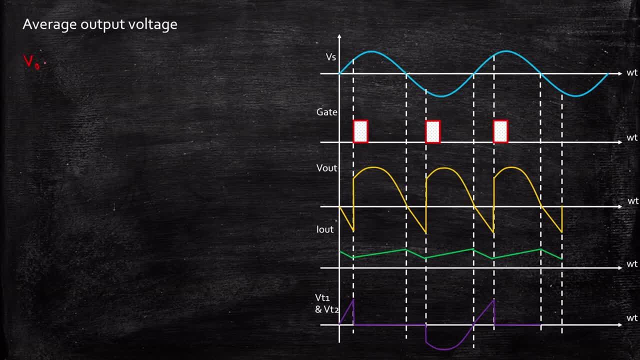 the expression So fundamentally by the definition of average output voltage, vout is equal to one by total time period, that is equal to one by pi in this case, And the integral, the average output voltage, we're considering only with respect to pi. 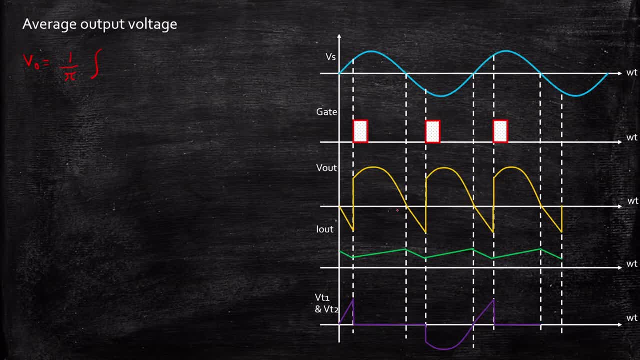 because the cycle is repeating continuously, isn't it? So, if you carefully observe here, this is pi plus alpha, And this is alpha. So the average output voltage for one cycle is starting at this point and descending at this point, So the lower limit will be alpha. 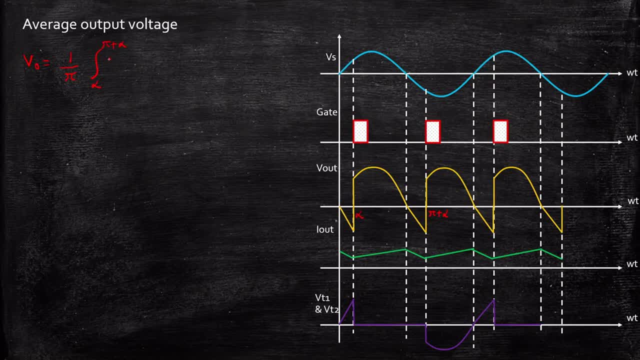 and the upper limit is pi plus alpha and we have vm sin omega t into d omega t. Now can we write vout? can we take vm outside? and when we integrate this we will be having minus cos omega t from alpha to pi plus alpha. Now vout is equal to vm by pi into minus of. 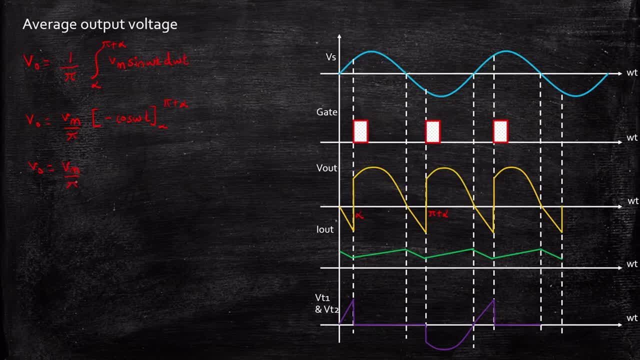 pi and it is pi plus alpha. Now we can write vout into sin omega t. Now vout is equal to vm by pi into minus of pi plus alpha of cos of upper limit, that is pi plus alpha. minus of minus will be plus, So you'll be. 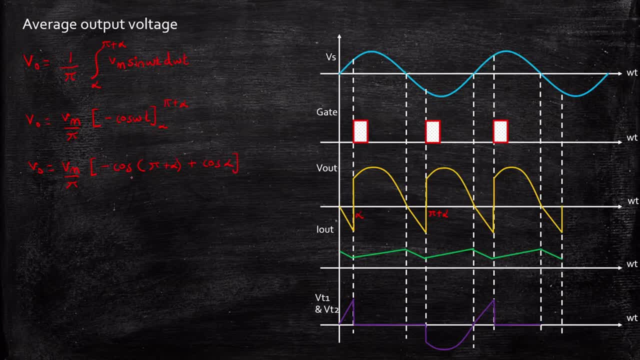 having cos alpha for the lower limits. So from the trigonometric functions we know that cos of pi plus alpha- this particular term can be written as minus cos alpha, So minus of minus will be plus cos alpha, So plus and plus will get added up. So we will. 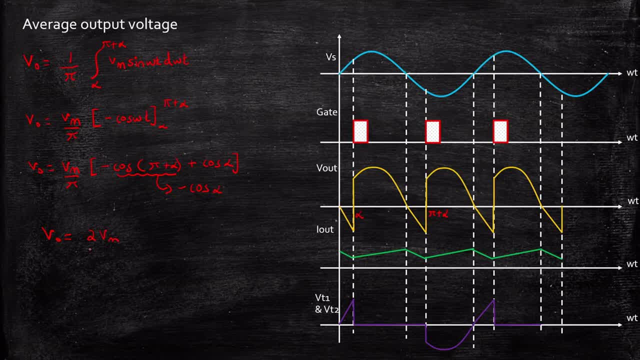 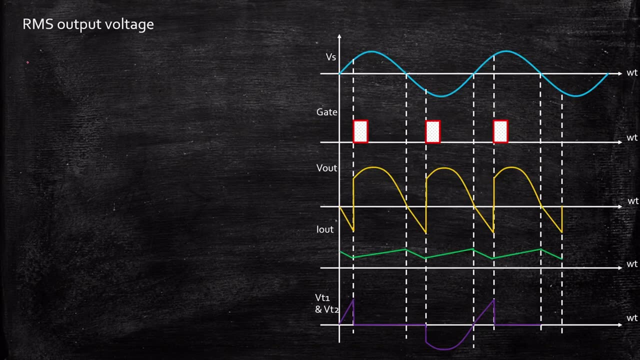 be left out. with Vout is equal to 2 times Vm by pi into cos alpha. This is the average output voltage expression. Now let's take a look at the RMS output voltage. Again, we will be deriving an expression for this Vout. RMS is given by fundamental definitions: square. 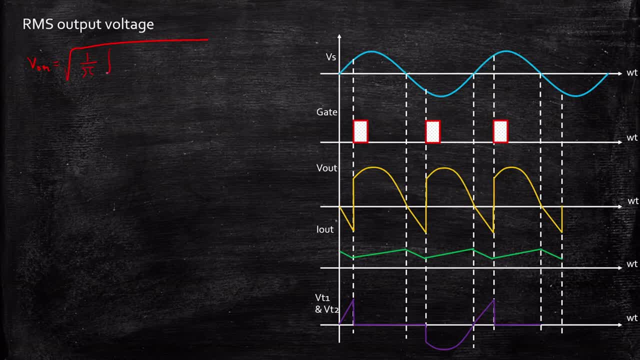 root of 1 by total time period, that is pi, and we have upper limit and lower limit, that is alpha to pi plus alpha, Because this starts from alpha and it remains till pi plus alpha. Vm square sin, square omega t into d omega t. So Vout RMS is equal to square root of. let us take Vm square outside. 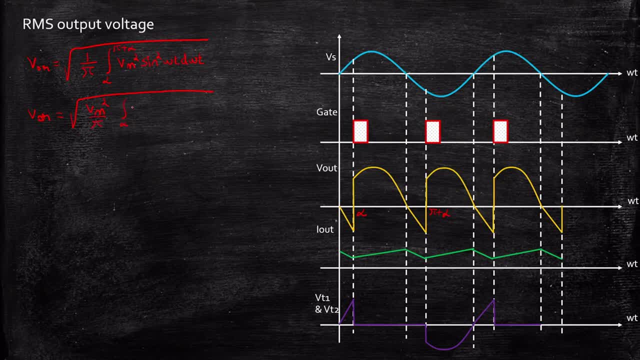 Vm square by pi into alpha to pi plus alpha Sin. square. omega t can be written as 1 minus cos 2. omega t whole divided by 2 into d. omega t Isn't it So Vout? RMS is equal to square root of Vm square by pi into applying the integral, that is 1 by 2. integral is omega. 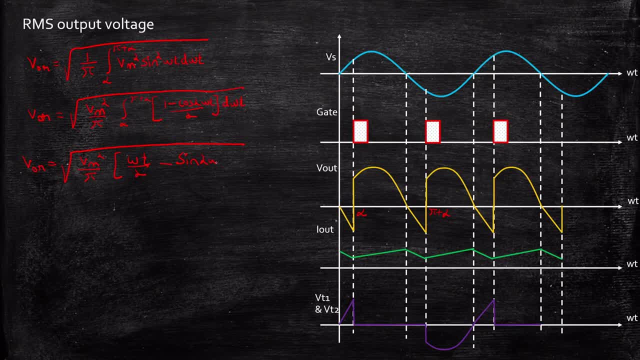 t by 2 minus cos 2. omega t integral is sin 2. omega t whole divided by 4 applying chain rule. so Vout RMS is equal to square root of Vm square by pi. so omega t by 2. we can write pi plus alpha applying the upper limit: whole divided by 2 minus sin of 2 times pi plus. 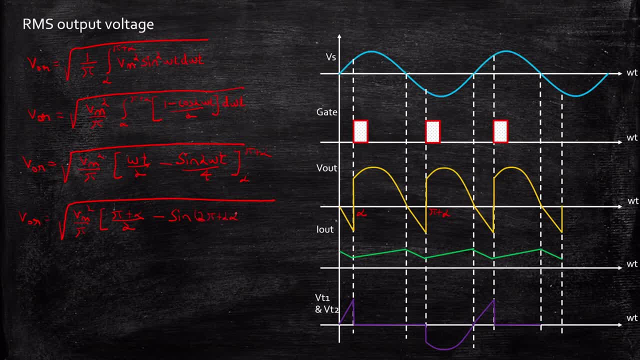 alpha, that is 2pi plus 2alpha. isn't it whole divided by 4 minus Great, Thank you. the lower limit of omega t by 2 is alpha. by 2 minus of minus will be plus, so we have sine. 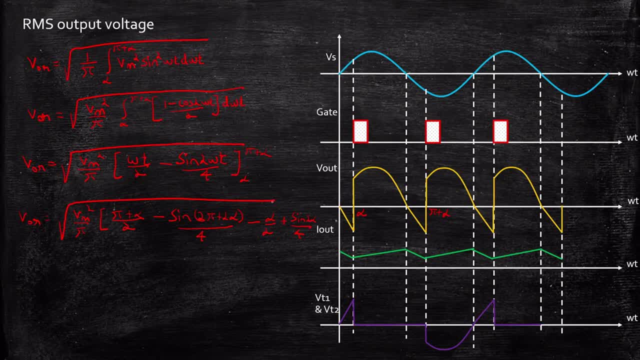 2 alpha by 4. now one important observation here: sine of 2 pi plus theta can be written as sine theta. so this can be written as sine of 2 pi plus 2 alpha can be written as sine 2 alpha, so replacing that sine 2 alpha by 4 and sine 2 alpha by 4 minus and plus here. 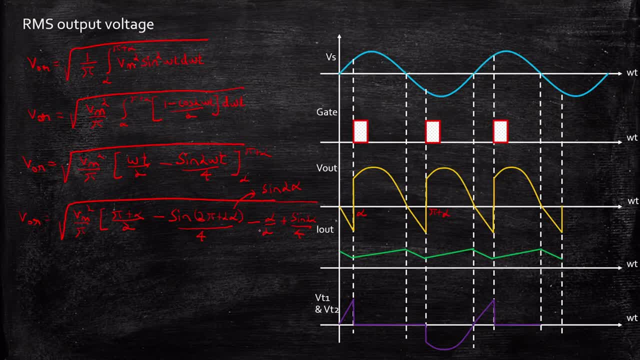 will get cancelled out. alpha by 2 plus alpha by 2 minus alpha by 2 will get cancelled out. pi and pi will get cancelled out, so we will be left out with vout. rms is equal to vm by root 2. this is the rms value of output voltage for an RL load for a single phase, fully controlled. 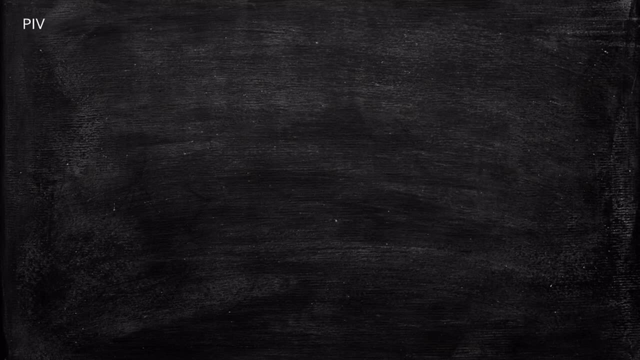 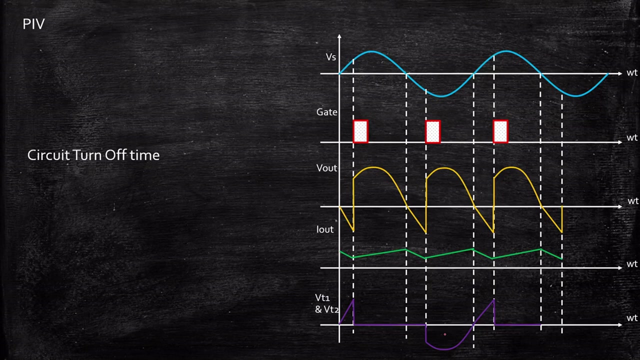 rectifier. now, what is the peak inverse voltage and circuit turn off time? so, if you carefully observe, the maximum negative voltage that is appearing across thyristor t1 and t2 is minus Vm, isn't it? so the peak inverse voltage, by its definition, is equal to minus Vm, but